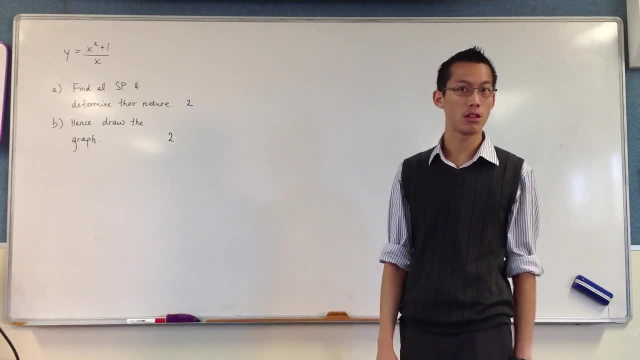 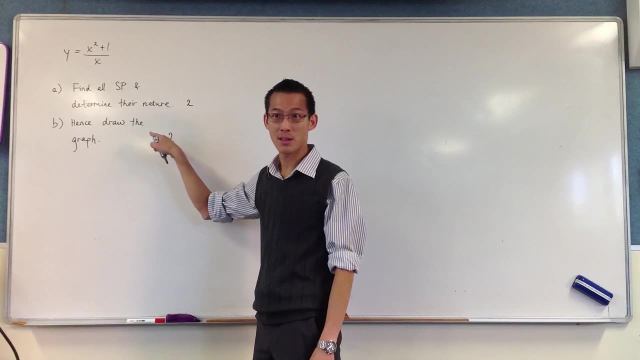 Typical question: Find the stationary points, determine their nature. then let's draw the graph Now, even though it doesn't say showing all features: blah, blah, blah, blah. See how it says: hence, Hence right. 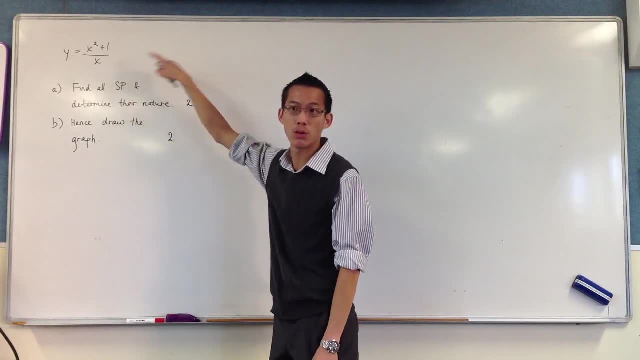 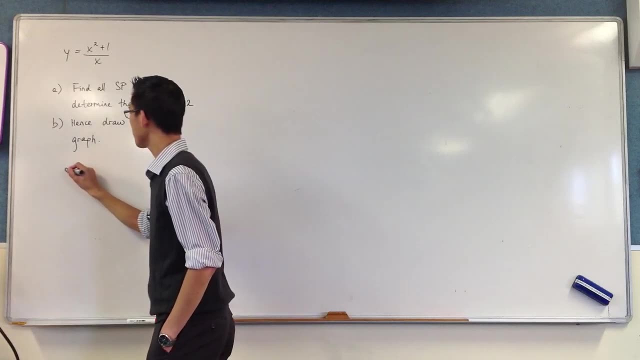 So, even though it's only worth two marks, they're expecting you to include all of the things from earlier parts of the question. all right, So let's give this a go. shall we Find all stationary points? What do I need to do to find stationary points? 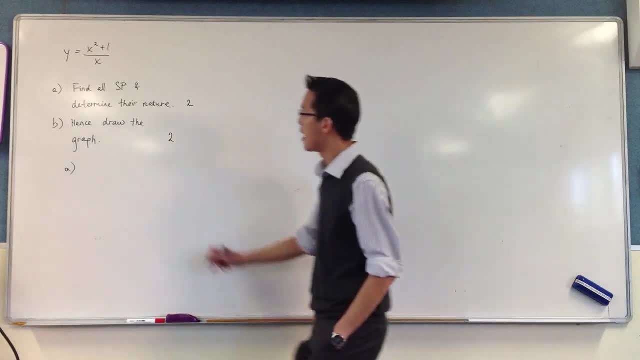 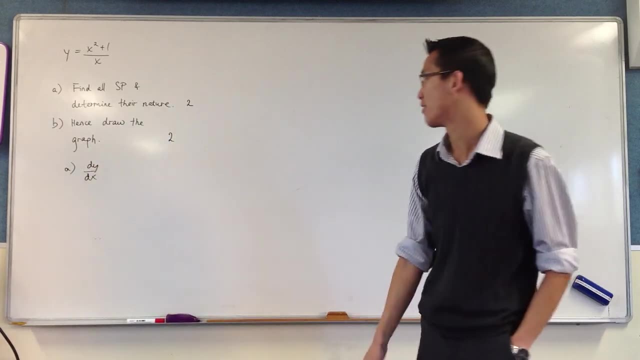 All right, differentiate, okay. Now I've also picked out this question because it's a classic error to make in it. right, What you've got is a quotient. so the instinct you've got, especially in an exam when you're under pressure- 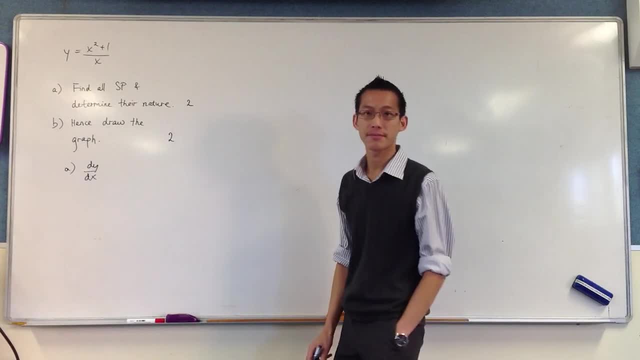 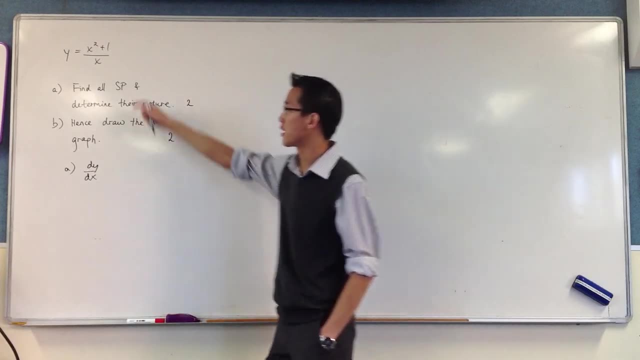 is: go to the quotient rule, right, But you shouldn't. why not? Because you can divide it up, okay, And then you just get two fractions which are really easy to deal with, rather than doing VU minus, sorry, VU. 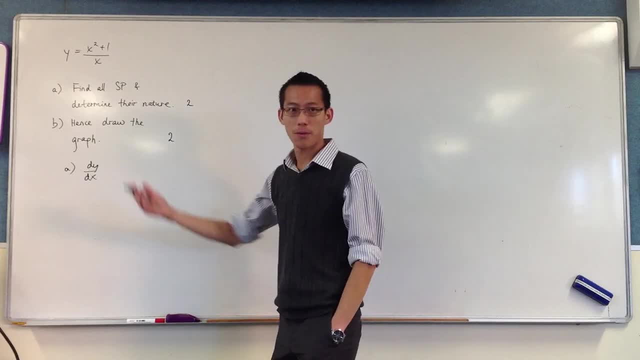 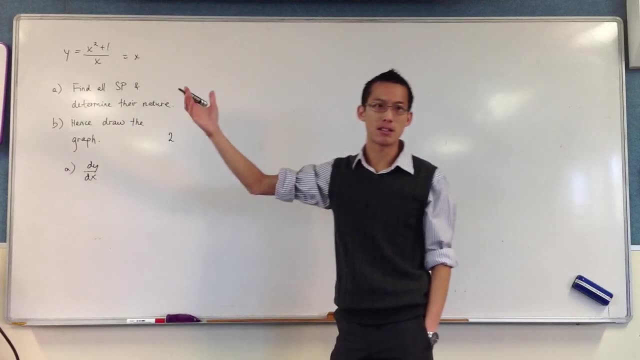 VU dash minus VU V dash on V squared, it'll be a disaster, okay. So how do I break apart X squared on X is just X and the other part's 1 over X. simple, That's a little more manageable, okay. 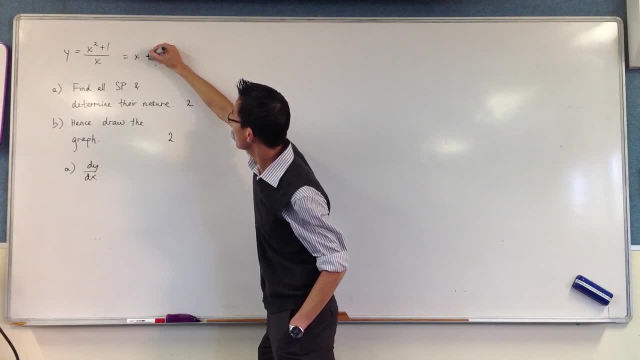 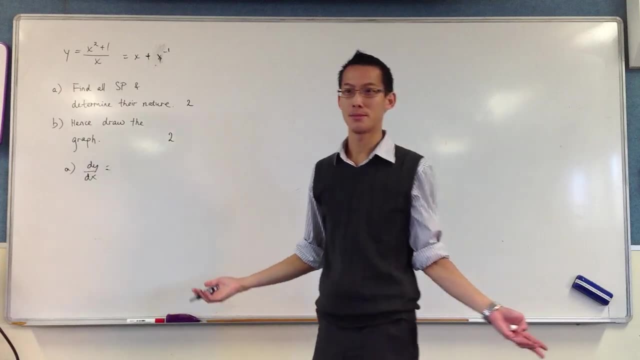 In fact, I might write this as X to the minus 1, because that'll help us when we differentiate. Okay, so derivative: Just take each piece one at a time. Derivative of X is 1.. Derivative of X to the minus 1.. 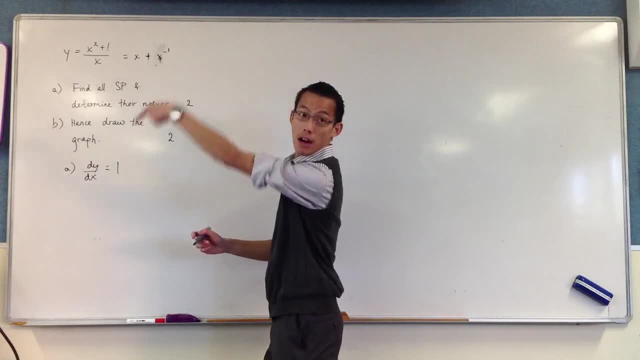 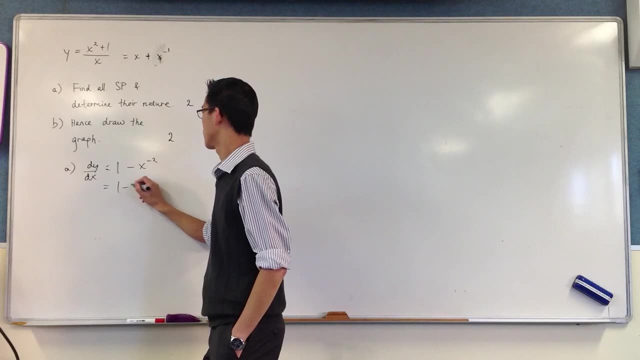 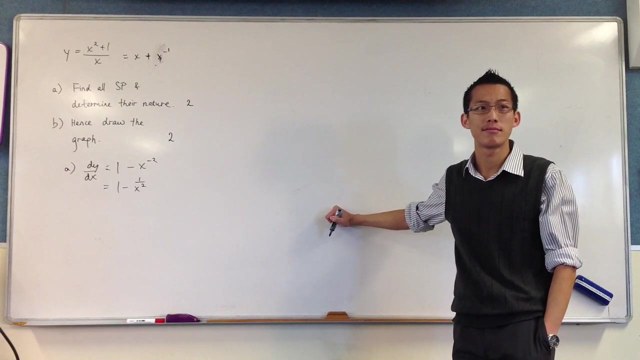 What do we do with it? Bring the power out the front, so minus, and then reduce the power by 1.. Okay, so far, so good. Now what? What do I do with this derivative? Good Now, by the way. please don't just say: 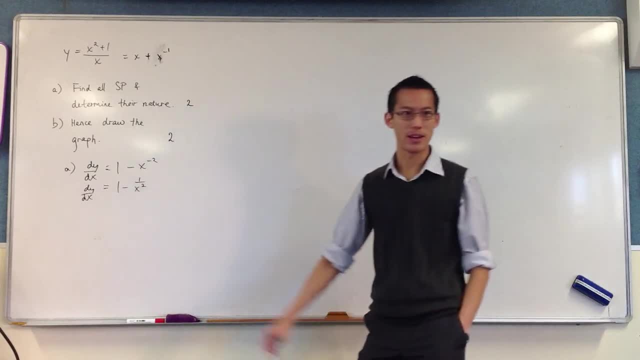 we've said this before. don't just go next. line 1 minus 1 on X squared is equal to 0,. okay, It's not, but we want it to be for a particular case, So put your logic in, okay. 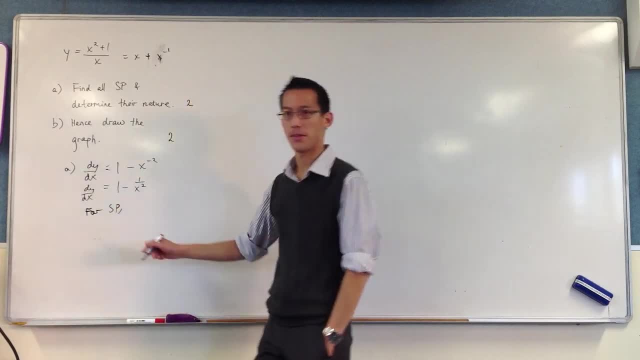 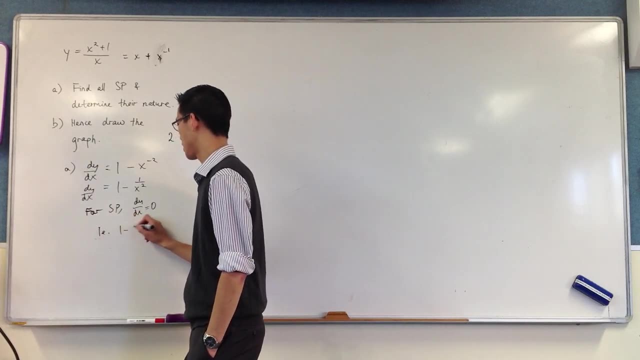 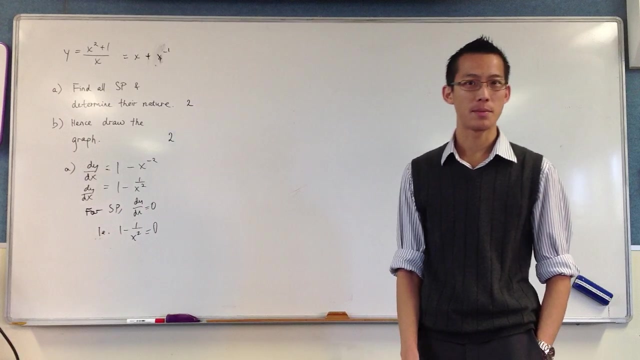 For stationary points. okay, the derivative is 0.. Okay, and what that means is this expression which we just worked out: that's equal to 0, okay, Can anyone tell me what the values are we're going to expect? 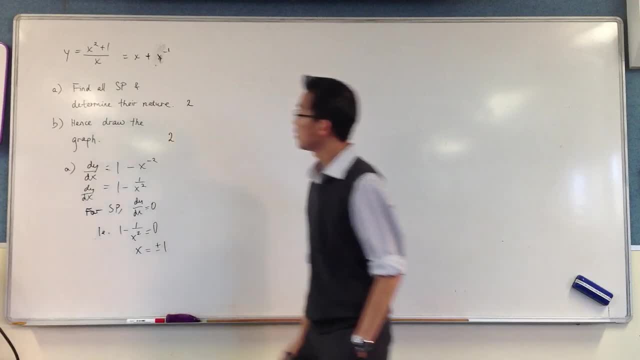 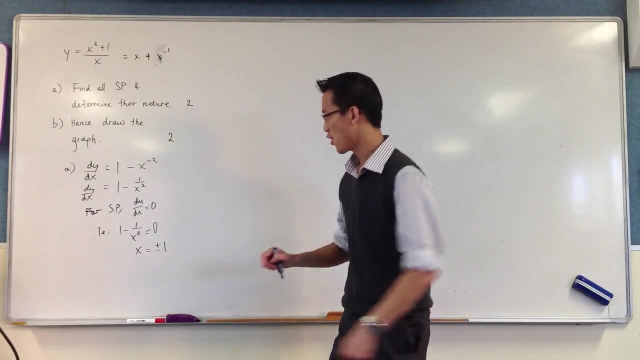 Good, Okay, Okay, Narrow the X values Now, find all stationary points and determine their nature, okay, So I've got a little more to go before I've actually found it. I know where it's X is which is horizontal. 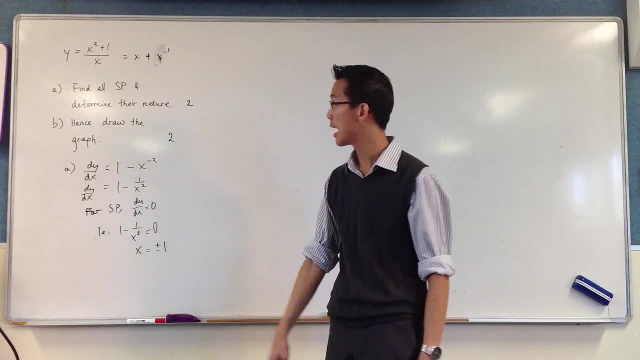 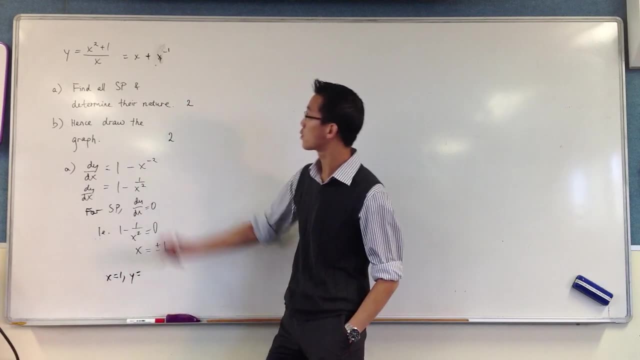 but I'm going to need to know where it's Y is okay. So how do I do that? Good, Okay. So when I say X equals 1, Y is going to be equal to 2? 1 plus 1.. 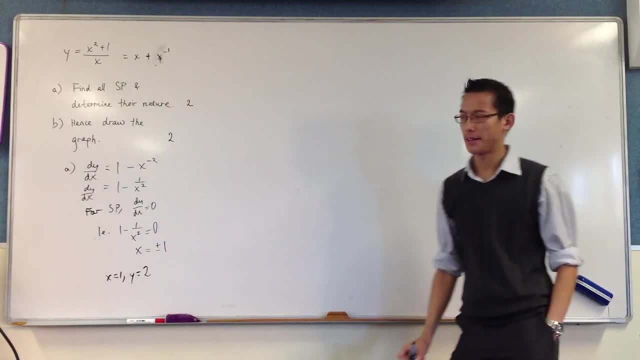 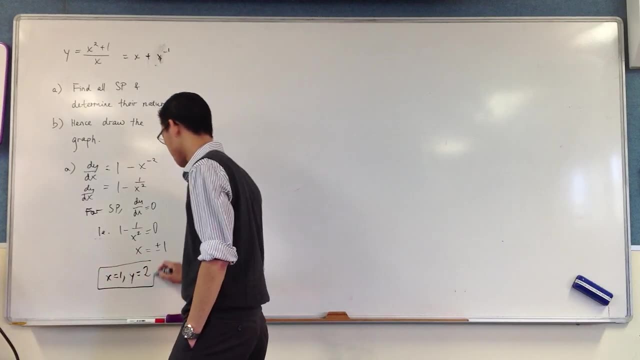 Do you have to show your full summing in and stuff? Oh my God. Okay, We will have to show sum for working, but you'll see later on. okay, So there's one of our stationary points, okay, And the other one, X, equals minus 1.. 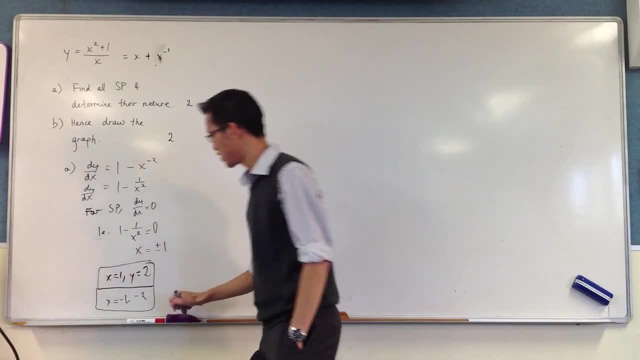 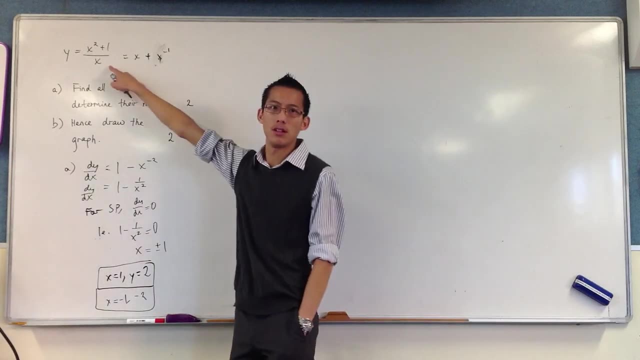 Minus 2.. Now, at this point you ought to be getting suspicious, because there's a lot of symmetry here, right, Which we should have picked up earlier. because what kind of function is this? Look at it carefully, Okay, Think back to further graphs from the lockers. 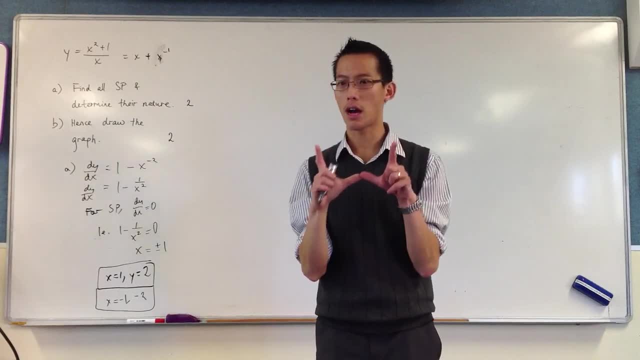 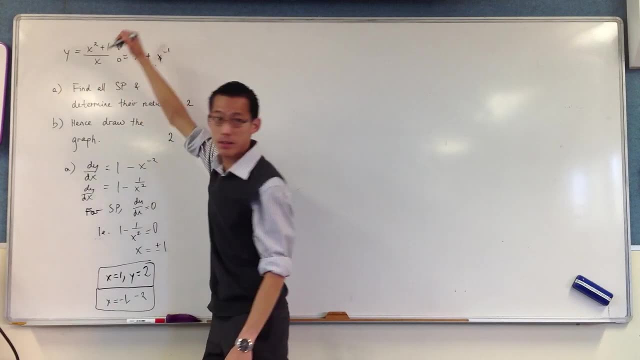 The top part: X squared plus 1.. Picture X squared plus 1.. What kind of function is it? It's even. The bottom is X which is odd. You have even or odd If you divide them or multiply them. 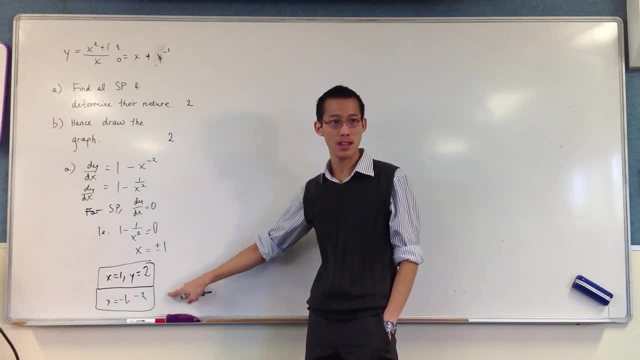 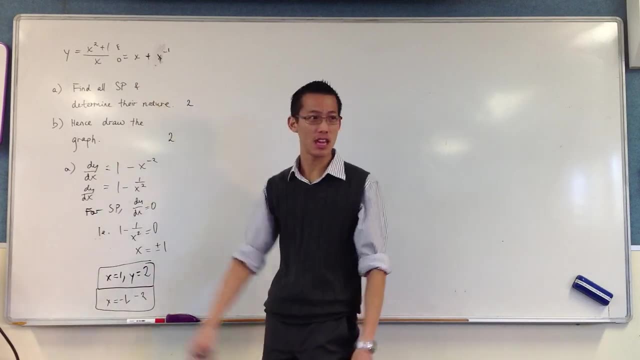 what you're going to get. the result is also odd. You see that 1, 2, right Minus 1, minus 2, okay, So you don't need to. I mean, it's not part of the question to say: 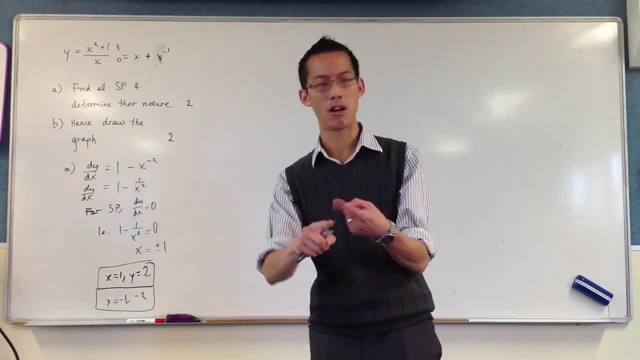 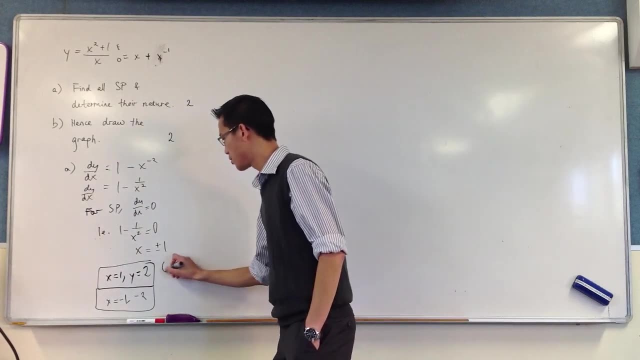 should. this is an odd function, right, But the whole reason we dwelled on odd and even functions is because they help you do things like this and it makes it faster. okay, All right, So 1, 2, and minus 1, minus 2.. 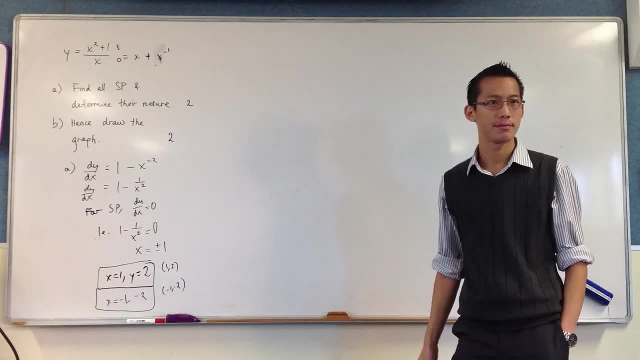 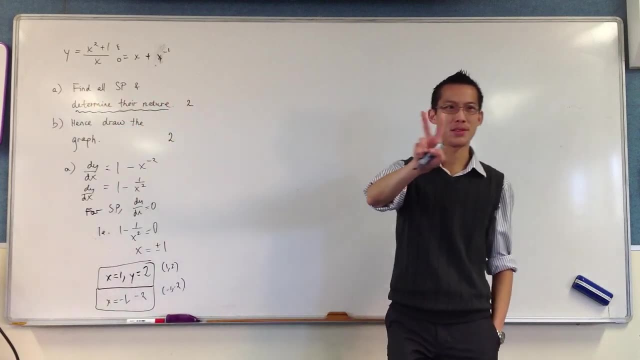 Okay, So now what I've found them. What do I have to do? Determine their nature. Okay, So, to determine their nature, you will remember we've got two options, right? What are the two ways we can go about this? 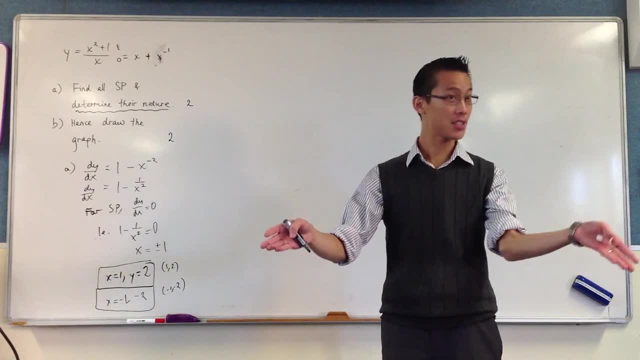 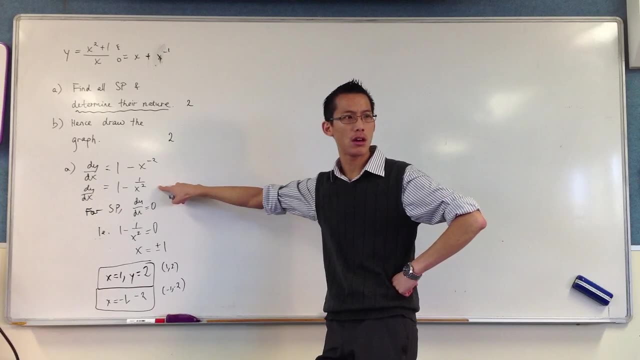 Second derivative: Okay, Second derivative or first derivative? okay, Now have a look at this function and this is its derivative. Which way do you think we should go? Should we use the first derivative and draw up the table, or should we do the second derivative? 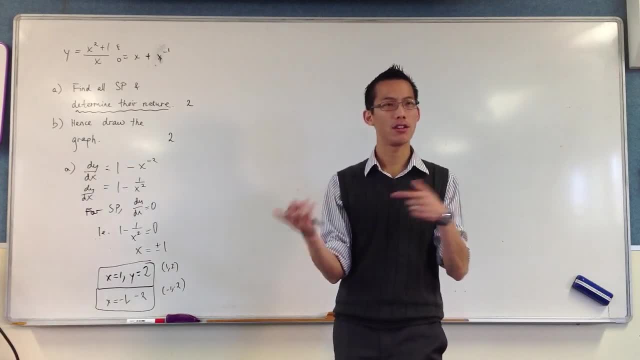 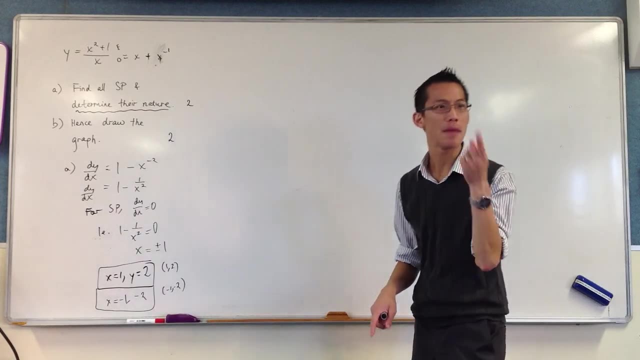 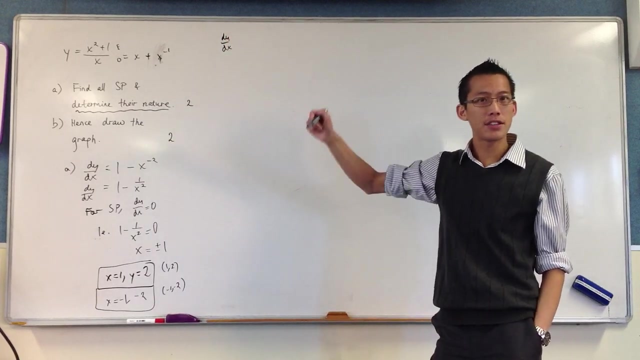 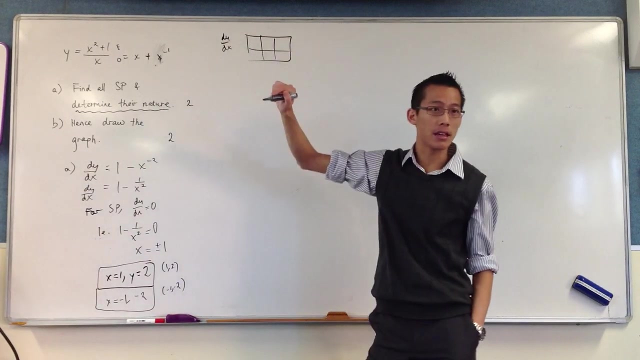 What's the thing that makes us choose? Let's just remember the way that you go about this. okay, If you're using the first derivative? okay, what you have to do is for each and every stationary point. okay, you have to test values on either side. okay, 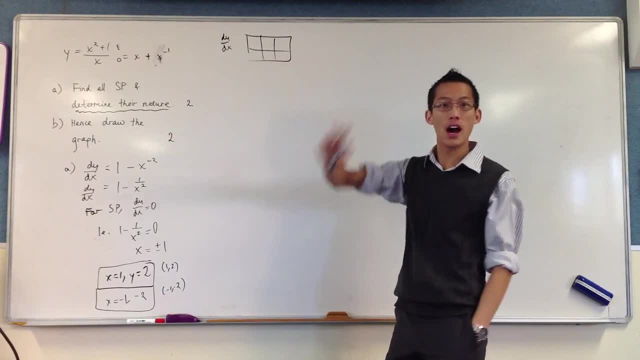 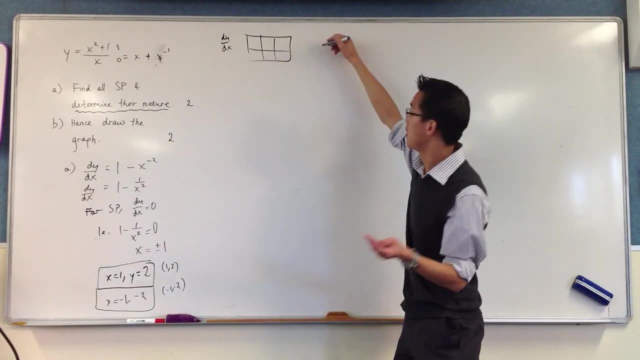 And then you want to show what the derivative is doing. It's going up and then going down, or vice versa. okay, And then you say it's a maximum or it's a minimum. okay, That's with first derivative right. 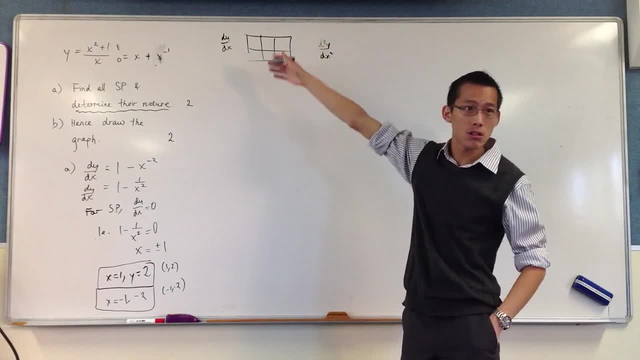 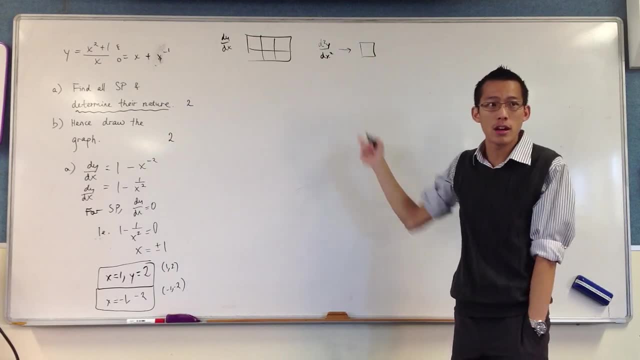 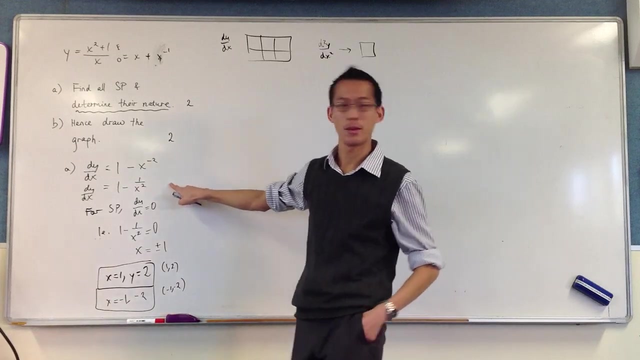 With second derivative. what do you do? You don't draw this table. What do you do? You just pop it in right, You just take one value, as it were. okay, So which is less work? This is less work, provided that differentiating is not hard, okay. 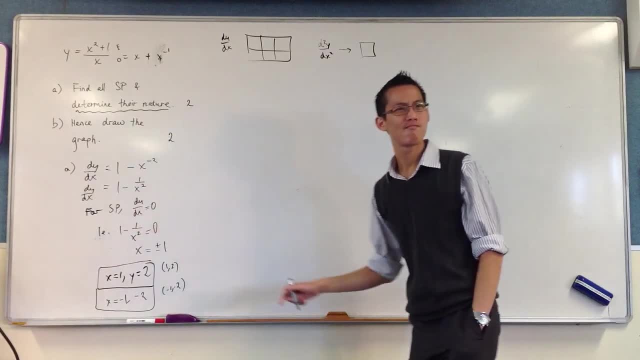 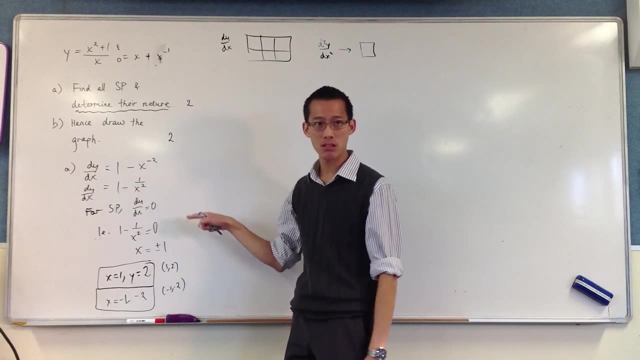 Now, is it hard to differentiate this again? It's not. it's not right, Because this 1 disappears. okay, This minus x to the minus 2, we just do the thing again. It's a polynomial. That's about the easiest thing to differentiate, apart from exponentials, okay. 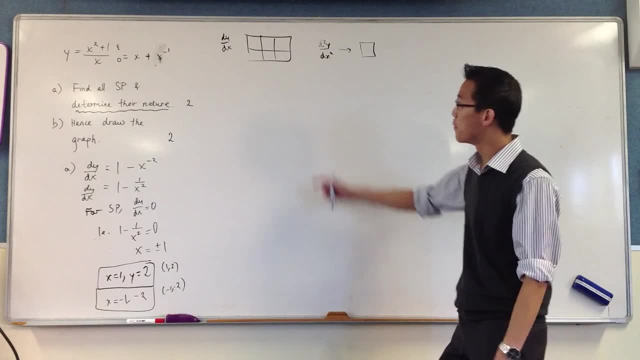 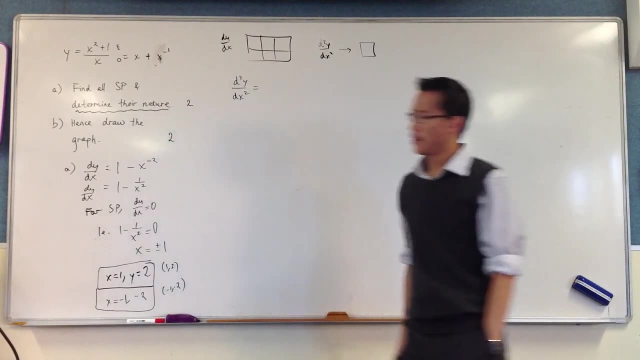 So I think we should elect to go the second derivative. all right, Remember, you can use either, But we're trying to save time here. all right, Yes, Okay, So I've got. I'm forgetting about the 1, because it just disappears. 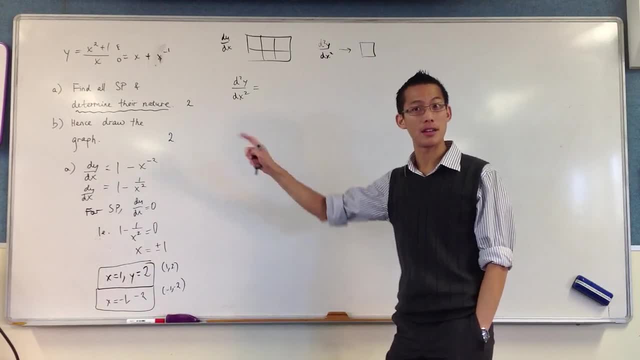 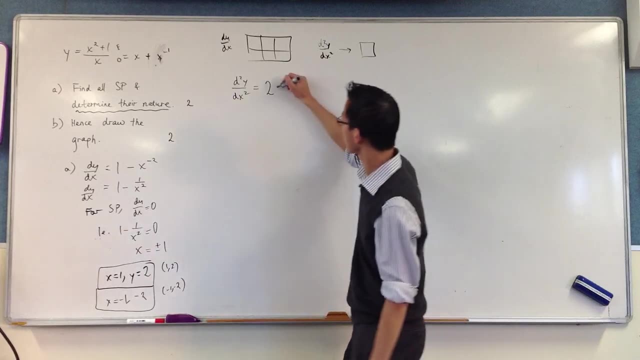 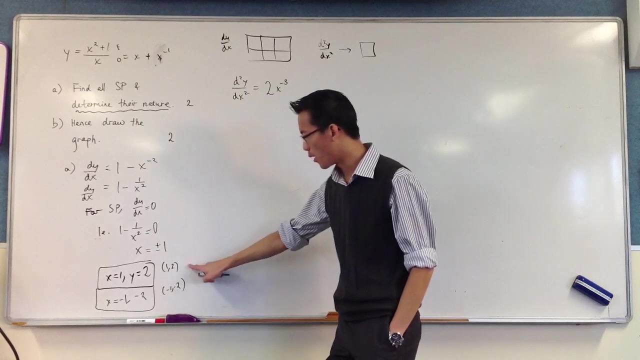 I've got minus x to the minus 2, okay, So bring the power down, Watch out for the double negative, okay, And then reduce the power by 1.. Okay, Now, what Good. So I've got my 1 and my minus 1, okay. 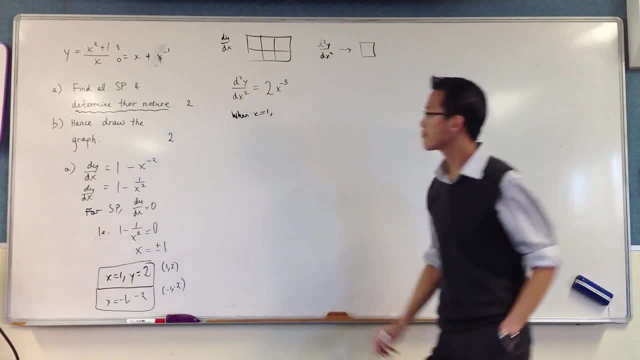 So I've got my 1.. So I've got minus 2, okay, So I've got my minus 2.. So I've got my minus 2 and my minus 1.. So I've got my minus 2 and my minus 1.. 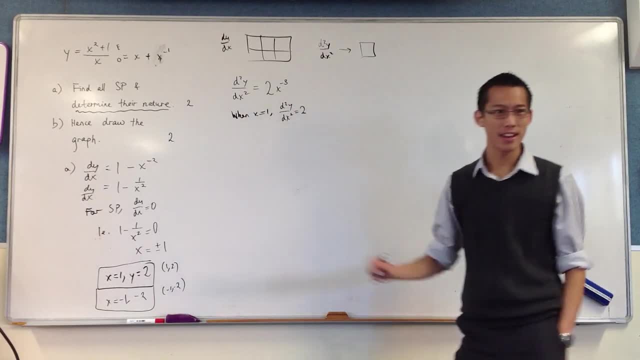 So what's the derivative of 2 over 1?? Well, x equals 1.. What's the second derivative? 2 over 1.. Good, Okay, Now hold on. What does this mean? Second derivative is positive. 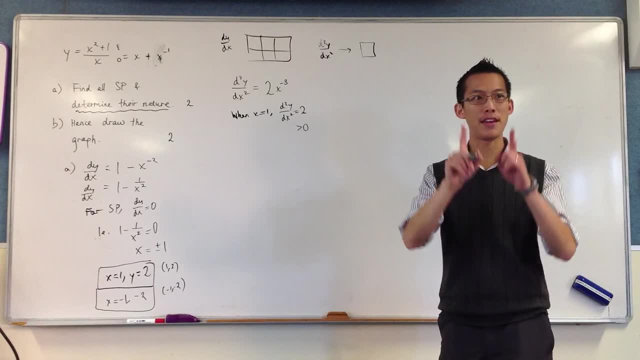 Which means it's facing up right. You can't remember what concave up looks like and what it means. You just draw it right And that means it's a local- sorry, I should say relative. So I've got my minus 1.. 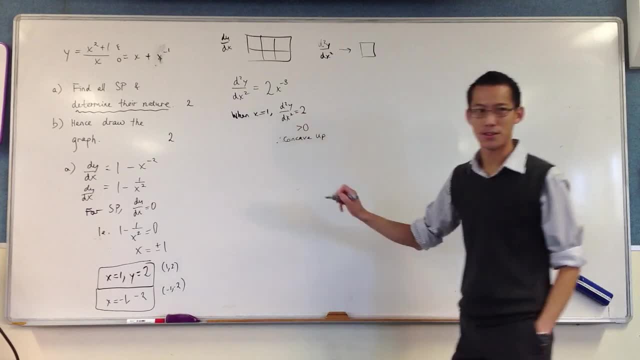 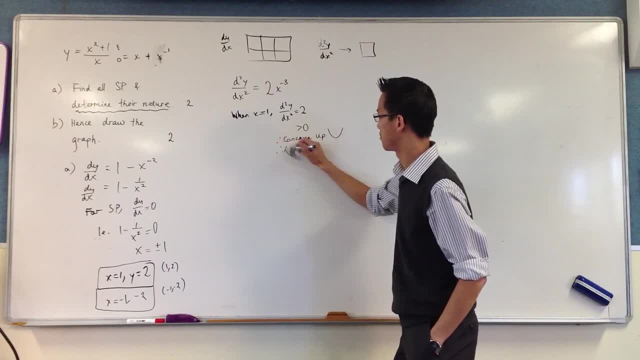 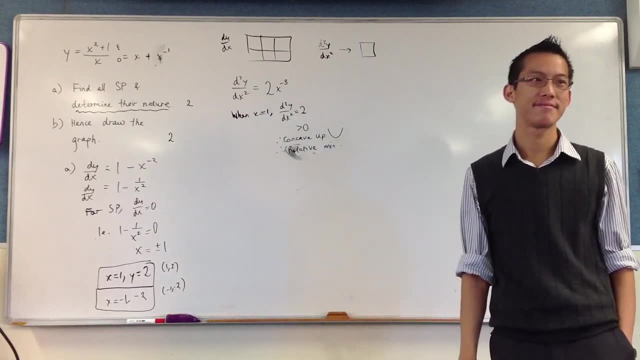 And that means it's a local. sorry, I should say relative. it's a relative minimum. You know the local and relative thing? Yeah, How do you get that? How do you know what's? It really doesn't matter. I'm saying relative because it's just policy. 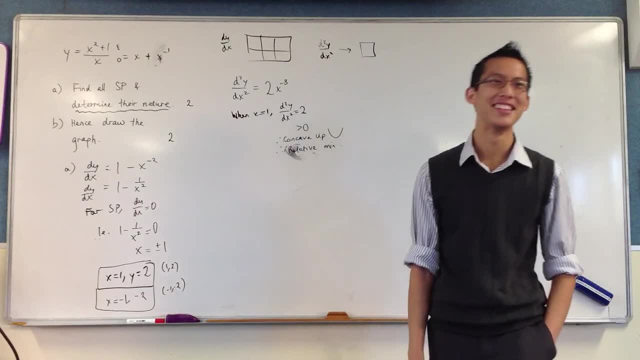 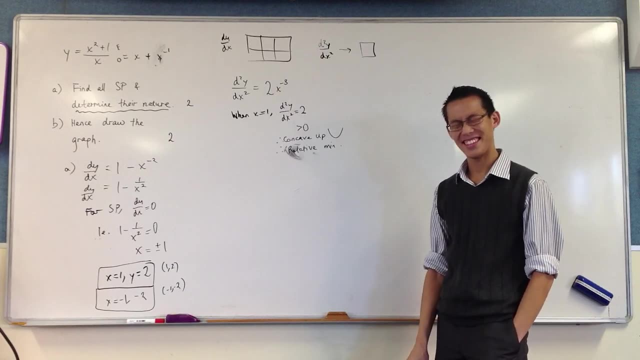 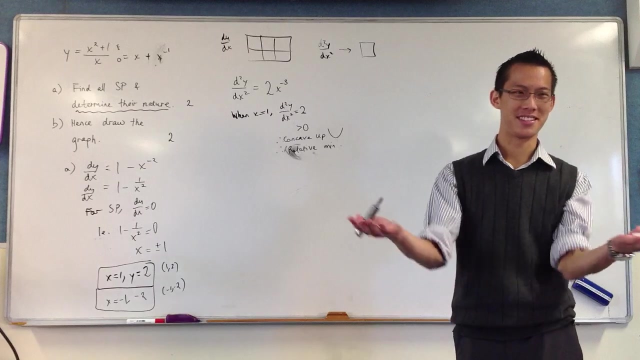 Are you allowed to say local and absolute? Local sometimes and relative other times? Are you allowed to say local and absolute? Oh, I see what you mean, Or something like that. Yeah, I suppose so, Though that seems a bit. I mean it's like: do you do the one question in millimetres and metres at the same time? 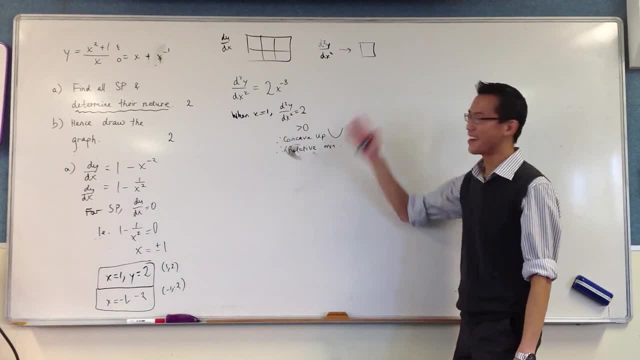 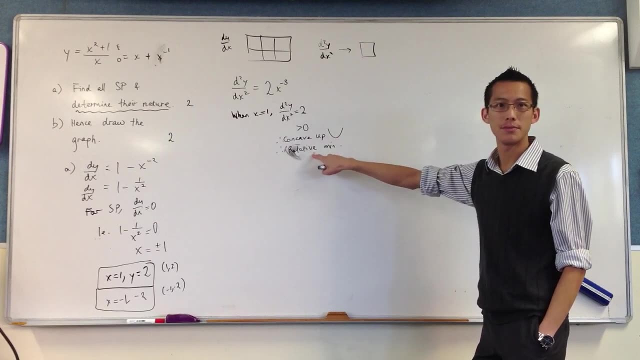 Oh, I suppose you could, but why would you? Anyway, okay, There's one. Now do you have to say it's concave-out? Can you go straight from here to here? The short answer is yes, you can. 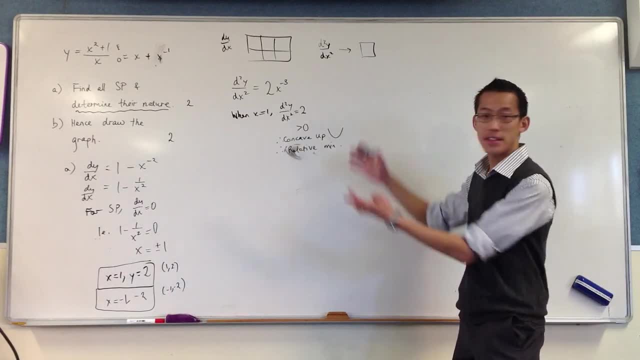 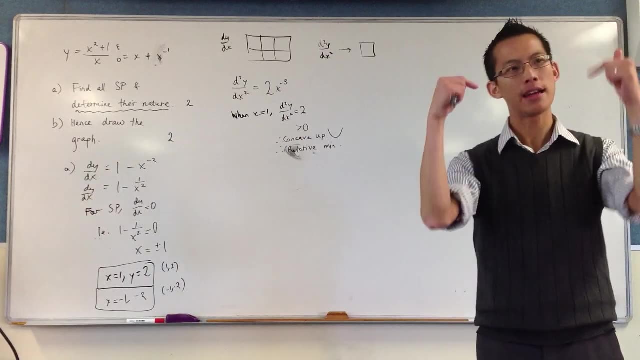 Does that mean you should do it? I don't think so. Okay, here's why. Remember: this is our first question. This is your first time assessing your ability to understand all of this. Okay, So what I'm looking for as a marker is not just: do they write down the right stuff? 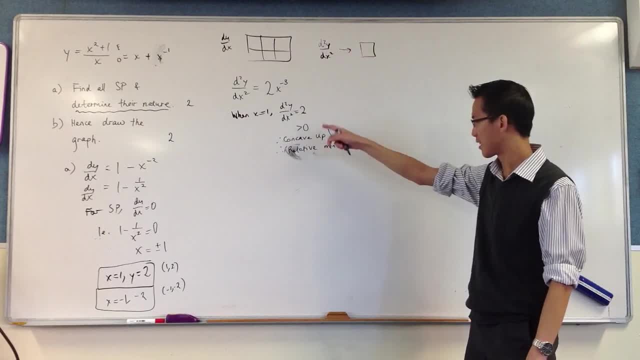 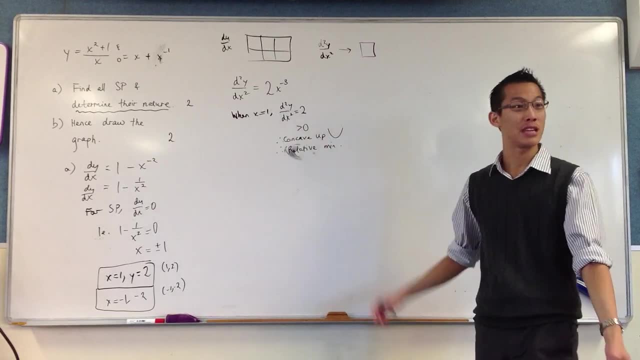 but can they demonstrate? they know what this all means. Okay, Like, this is greater than zero. so what Does that indicate? Okay, Why is it a relative minimum? Is it just like because a maths teacher said so? No, it's because it indicates this geometric feature, which is a minimum right. 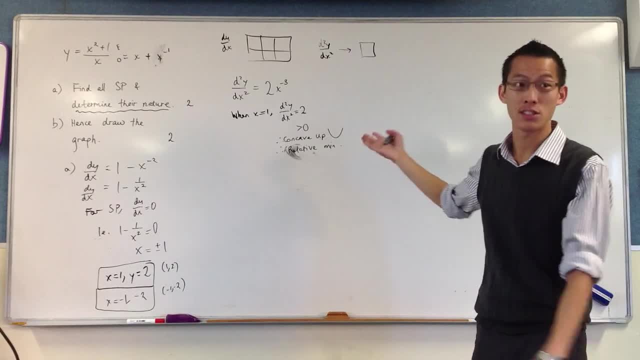 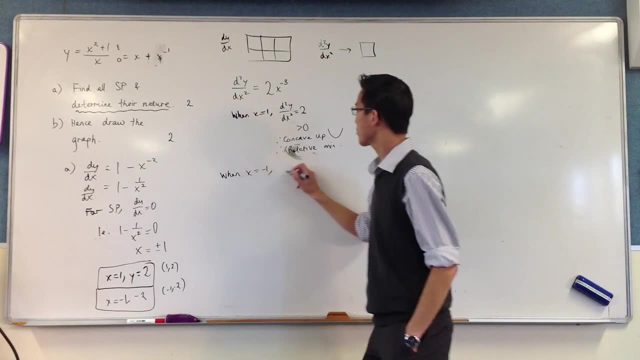 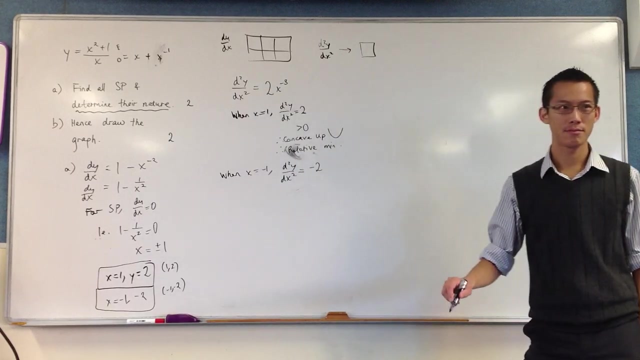 You can see it looks like a minimum right, So that's why I write it. I mean, I've been doing this for years and I still write it. Okay, I've got to do it for the other one. Okay, When x equals minus one, the second derivative is okay. odd function. 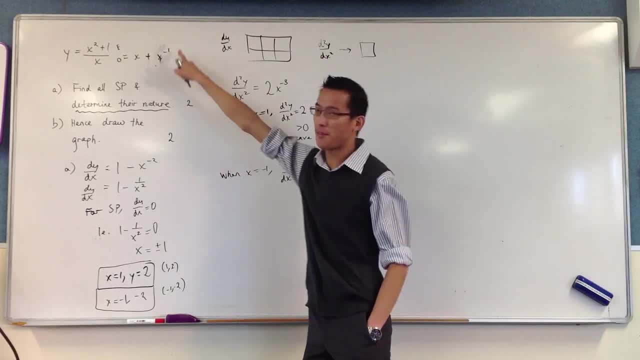 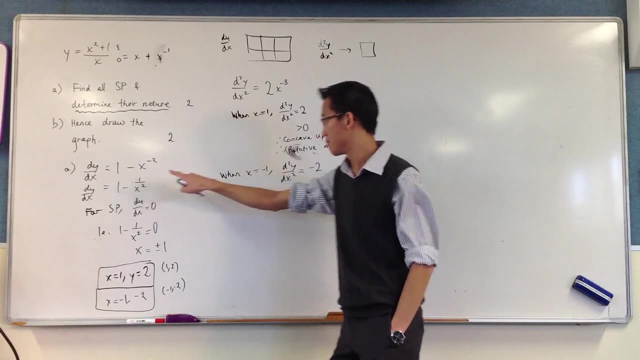 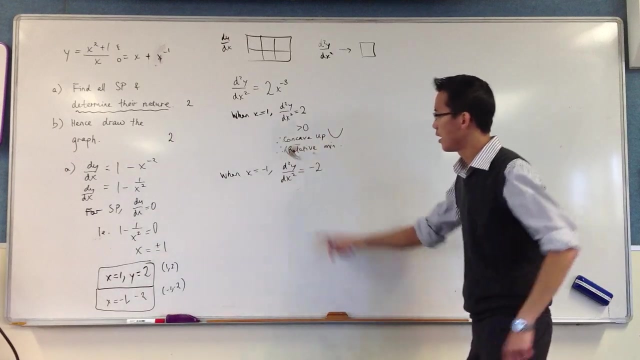 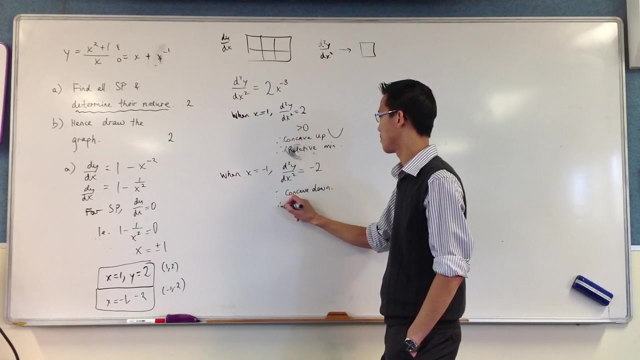 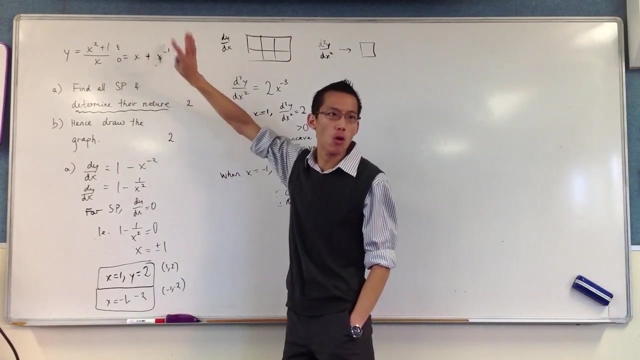 By the way, did you notice odd function right? First derivative is even x squared. Second derivative is back to odd. Okay, I appreciate you flipped between odd and even. Anyway, So this is concave down. All right Now, since this is a question all on its own. okay, you should actually conclude this question. 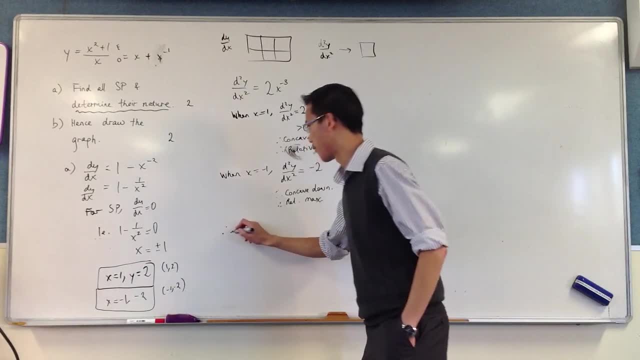 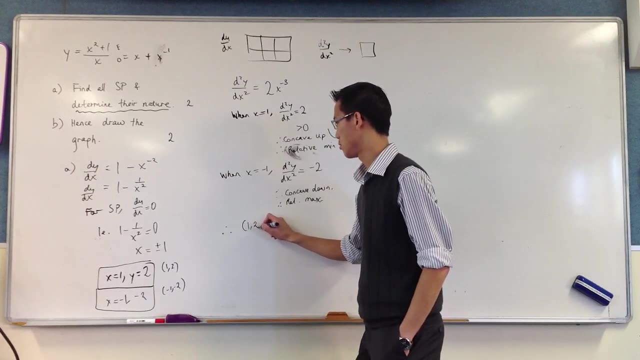 and actually have a sentence right. So you would say therefore, okay, I've got these two stationary points and I'm going to say what their nature is right. So I'd say one, two is a, which one was this one? 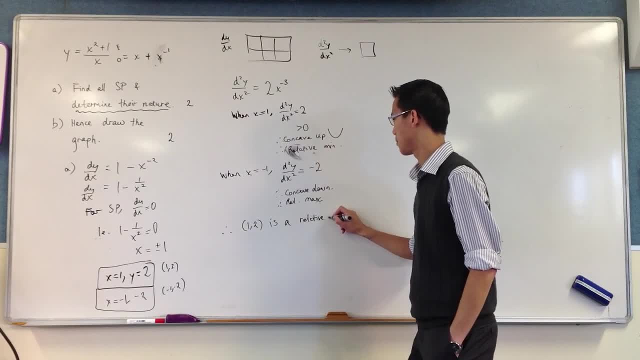 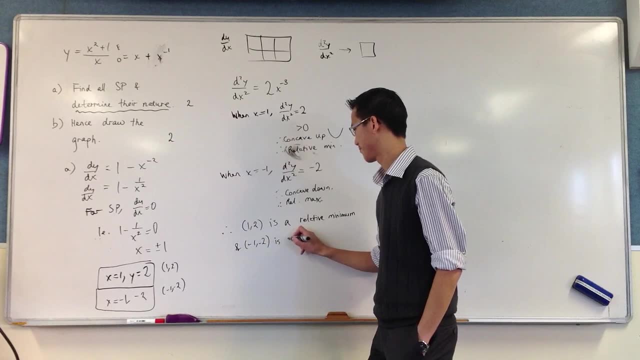 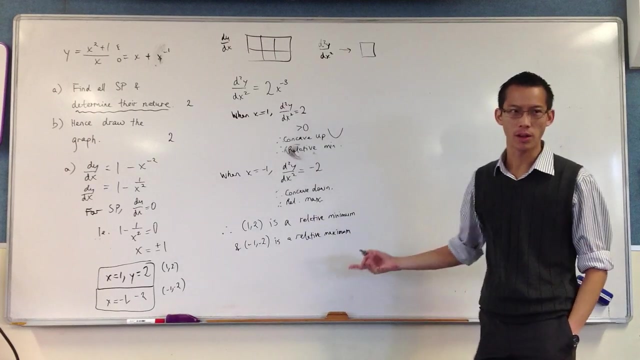 This one Is a relative minimum, And the other one is the other thing. If you're pressing times, is that anything about your? No, It's one of those things which the information is there. However, with something like this, I think it's particularly valuable, because you can. 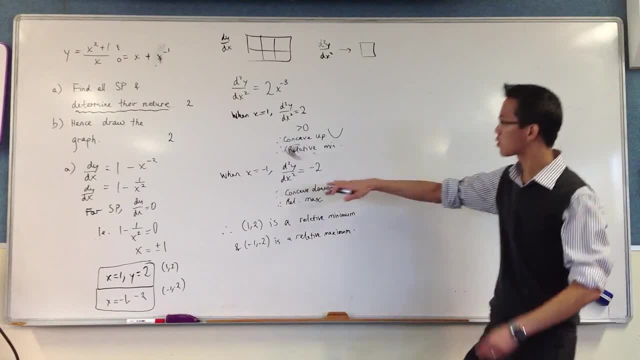 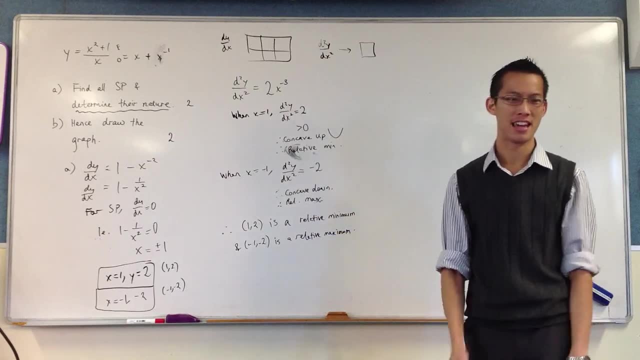 see that all of this actual information which is my answer, it's sort of scattered throughout all of my work. So, as you don't want to give extra work to the market, try and find your stuff and fail to find it and say this is not worth what it should be. 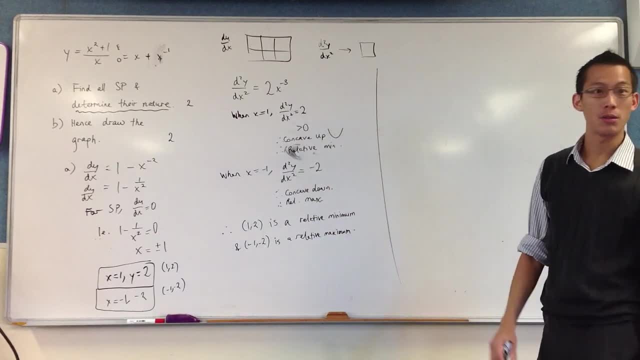 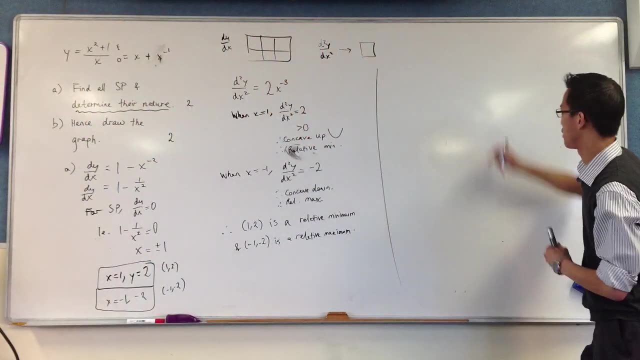 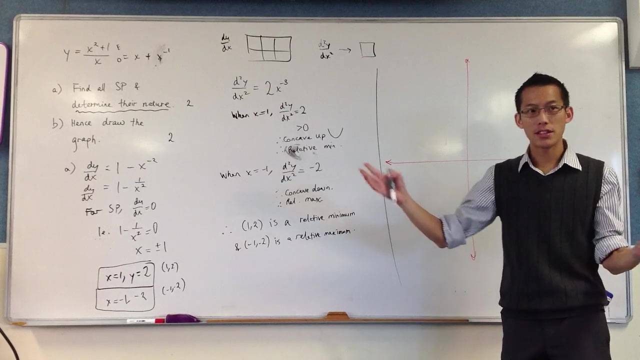 Okay, Right, Let's graph it, shall we? You've got. I need another color. Who's graphed it already? Anyone? Yeah, Okay, good, This will be quick. The first thing you do is take the information you've already got and plot it on there. 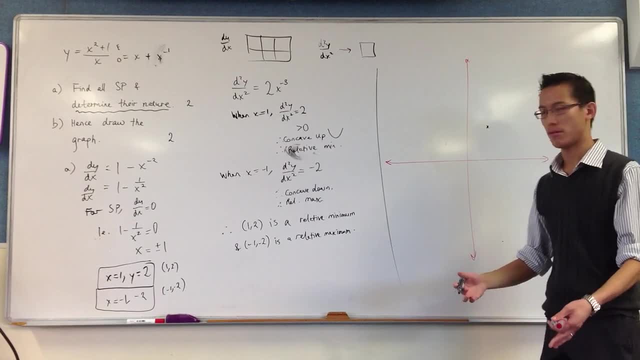 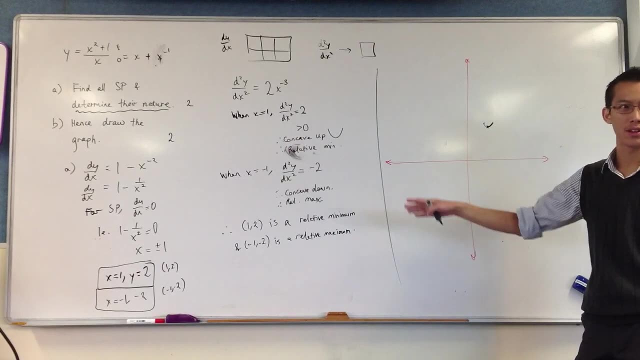 So one, two up here and it's going to be a minimum. So I'm expecting it to come up like that. And of course I'm actually not going to worry about the other side, because once I've got this side and I know what it looks like, it's a non-function. 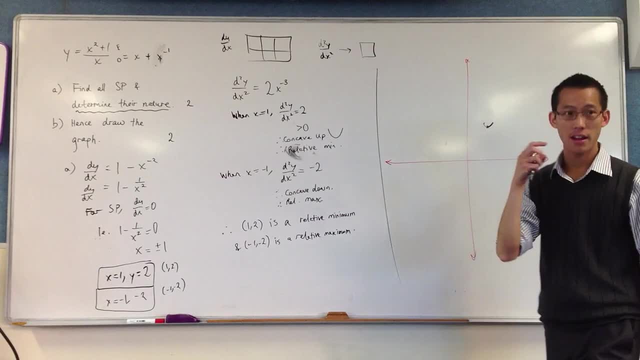 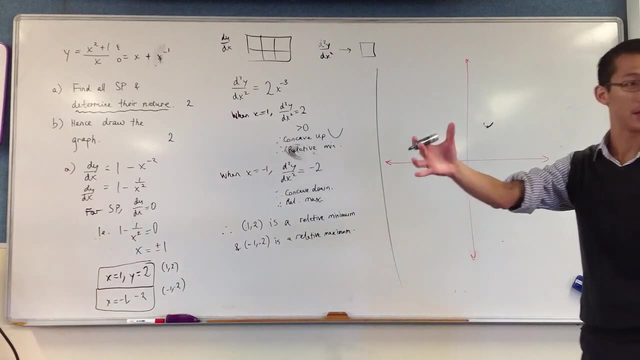 So I'm just going to draw it across the other way. All right, Apart from our calculus, what other features do we know about this thing? Good, Now, that's the kind of graph it is. What kinds of important features does our hyperbola have?